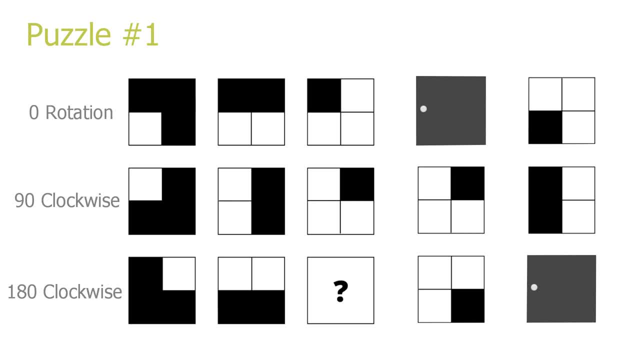 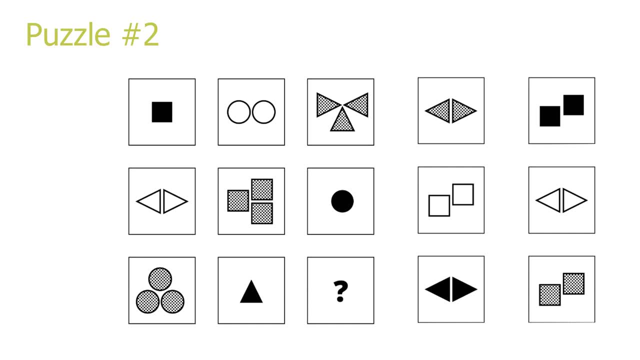 our correct answer. Rotating picture 6, 90 degrees clockwise gives 5 as the correct solution. Puzzle number 2.. This is a diagonal puzzle on both diagonals. First let's look at the top left to bottom right diagonal. Here we see that in that green diagonal we also have some points on the left side of. 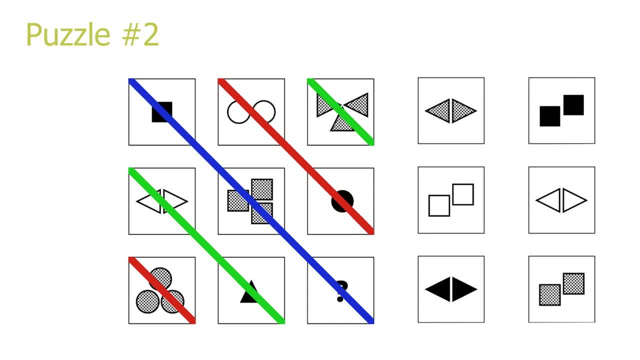 the right diagonal. These points on the left are theがとうCoolStyle Heilman, and it is very diagonals: the triangle repeat. on the red diagonals the circles repeat and on the blue diagonal the squares repeat. Our answer is in the blue diagonal. so we know that our 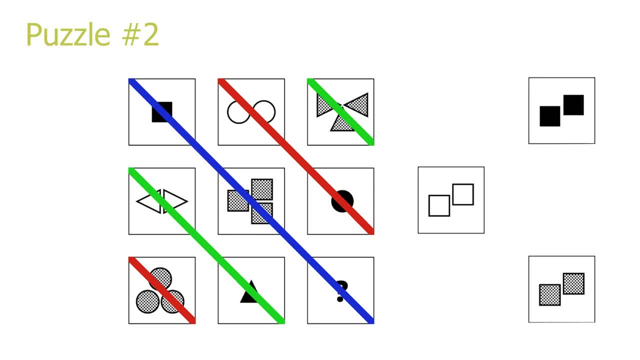 answer has to be a square. This leaves answer 2, 3 or 6 as the correct solution. Now let's look at the top right to bottom left diagonal First. on the green diagonals we see that the black inside and 1 shape repeats. On the red diagonal we see that white inside. 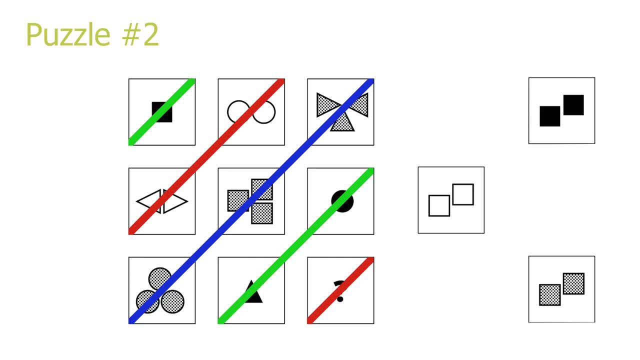 with 2 shapes repeat and on the blue diagonal we see that 3 shapes with a checkerboard pattern inside repeats. Our answer is in the red diagonal. so 2 squares with white inside is the correct answer. 3 is the correct solution. 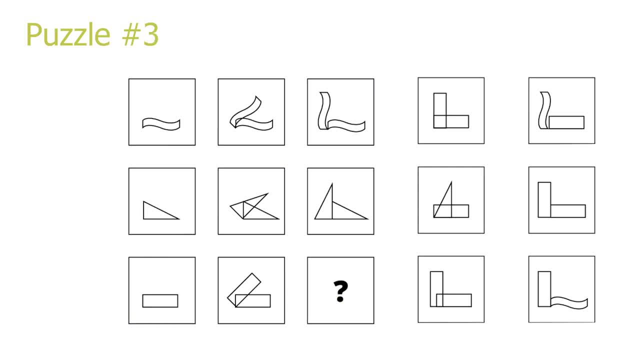 Puzzle number 3.. This is a row puzzle. The first thing I would like to point out are these points: These are the points of rotation, where the shapes are rotated around. So if we look at row 1, we see that the first picture is rotated 45 degrees counterclockwise around. 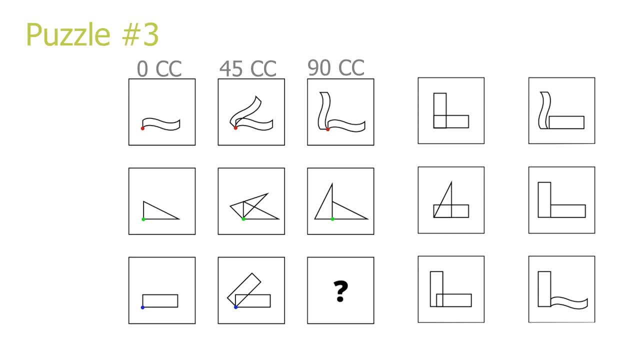 this point. So we add the whole thing on top of picture 1 to produce picture 2.. To produce the third picture, we just have to rotate the first picture 90 degrees counterclockwise and add it on top of itself, So, basing ourselves on the last row. we take the first picture, rotate it 90 degrees counterclockwise. 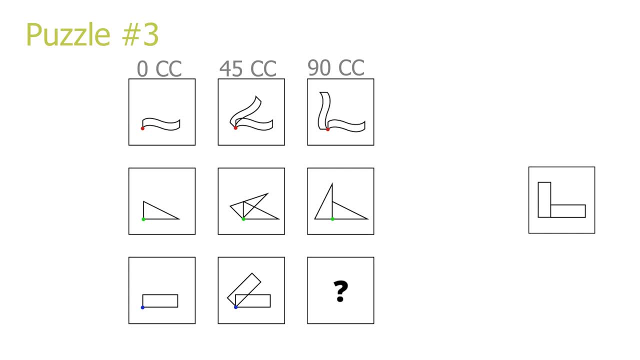 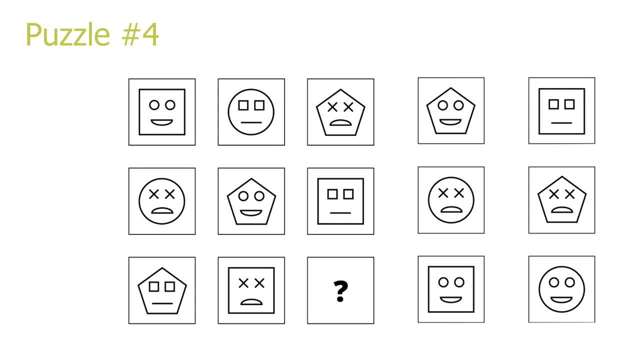 and add it on top of itself. So our answer would be a lying rectangle with a standing rectangle on the left side of it. 4 is the correct solution. Puzzle number 4.. This is a diagonal puzzle. In the top left to bottom right diagonal. we have a repetition of the eyes and mouth. 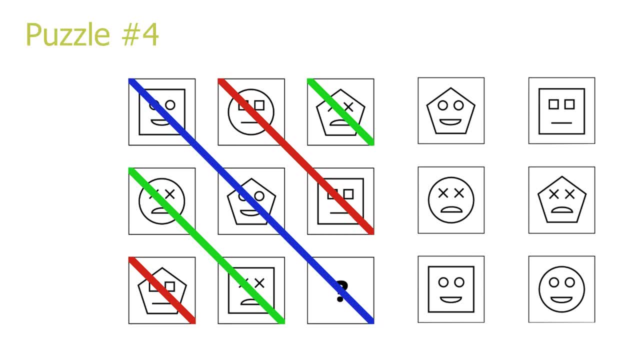 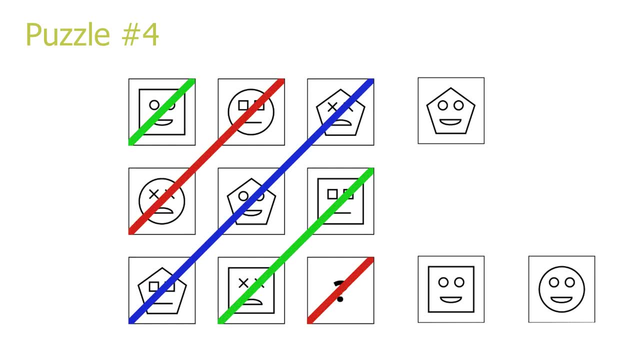 of the smiley fish cases. On the blue diagonal, which our answer is in, we have circle eyes and a smiling mouth. This leaves 1,, 5 or 6 as the correct solution. On the top right to bottom left diagonal, we have a repetition of the head shape. 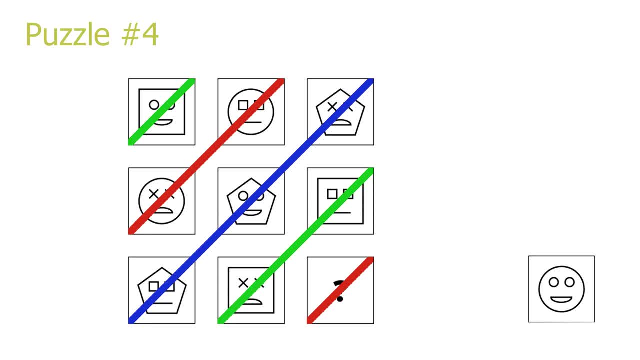 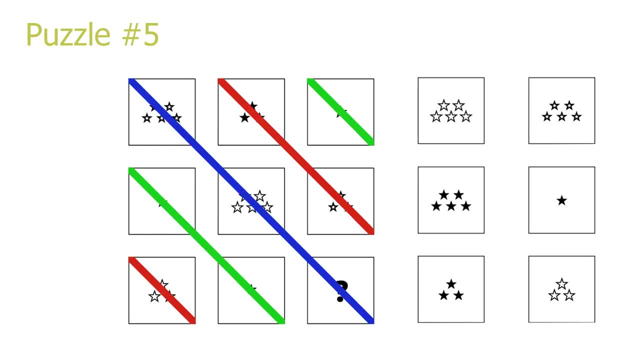 On the red diagonal, which our answer is in, we have a repetition of the circle head shape, which leaves 6 as the correct solution. Puzzle 5.. Another diagonal puzzle: Top left to bottom, right diagonal, we have a repetition of the amount of stars. 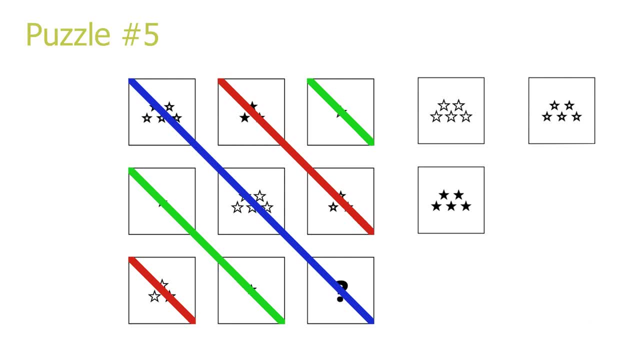 Our answer is in the blue diagonal. therefore, our answer has 5 stars. This leaves 1,, 2 or 3 as the correct solution On the top right to bottom left diagonal. we have a repetition on the color. Our answer is in the red diagonal, where every star is fully black inside. therefore, our 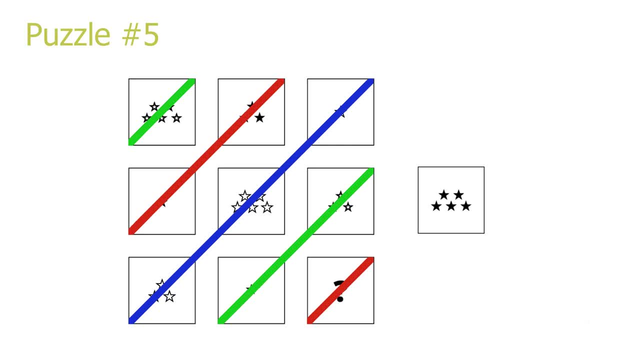 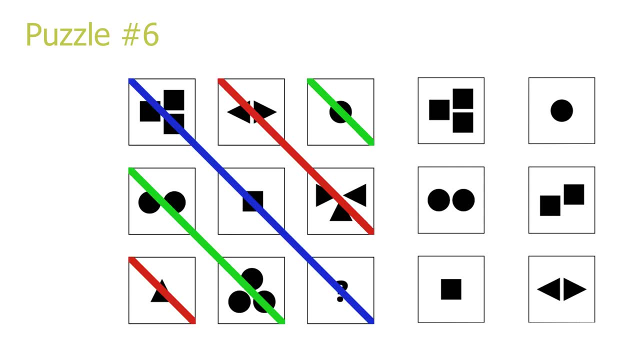 answer is 5. fully black stars: 3 is the correct solution. Puzzle 6. A diagonal puzzle: Top left to bottom, right diagonal. we have a repetition of the squares on the main blue diagonal. This leads to 1,, 4 or 5 as the correct solution. 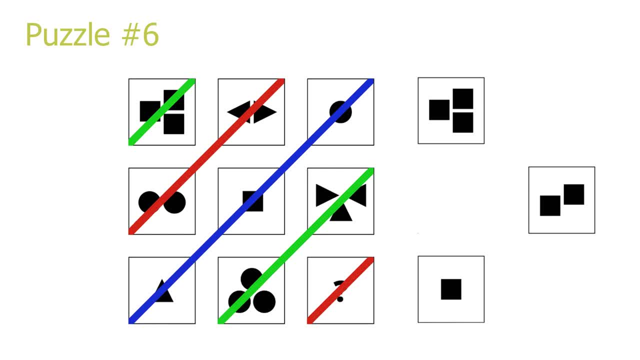 On the top right to bottom left diagonal, we have a repetition on the amount of shapes. On the red diagonal, we have 2 shapes repeating, leading to our answer being 2 squares 4 is the correct solution. Puzzle 7.. This is a diagonal puzzle. 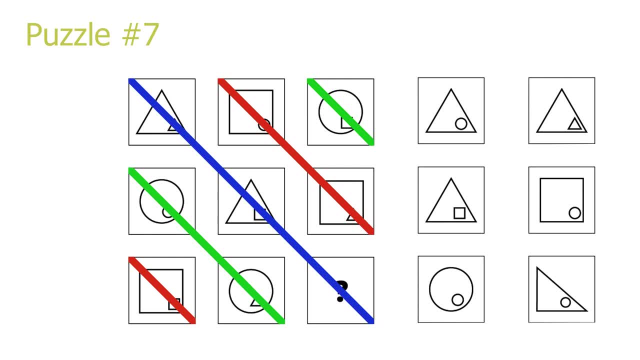 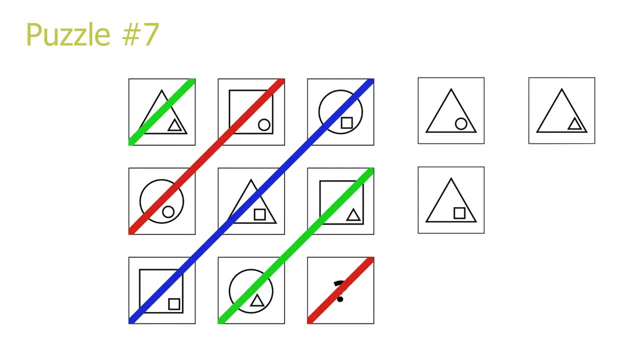 On the top left to bottom right diagonal, we have a repetition of the main shape, which is a triangle in the case of the main blue diagonal, this leaves 1,, 2 or 3 as the correct solution. On the top right to bottom left diagonal, we have a repetition of the smaller shape. 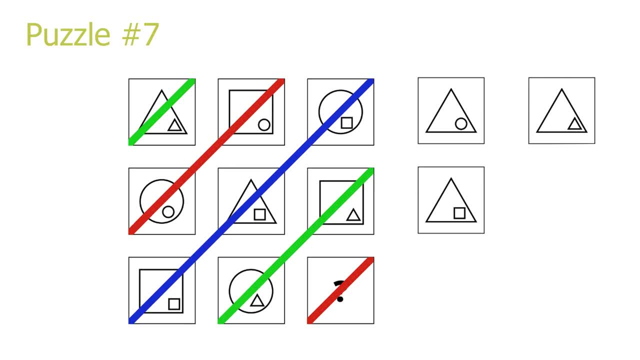 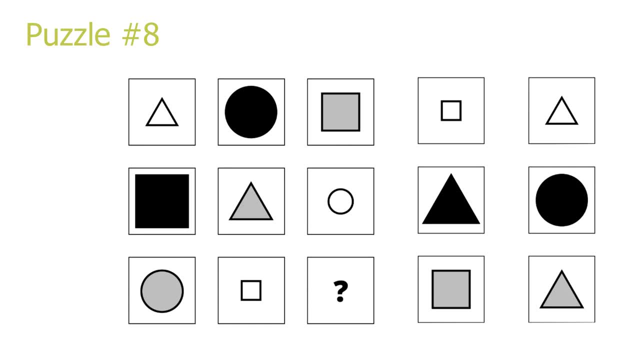 inside of the main shape, which is a circle in the case of the red diagonals. So our answer is a triangle with a circle inside of it. One is the correct solution. Puzzle number 8, another diagonal puzzle: On the top left to bottom right diagonal, we have triangles repeating on the main diagonal. 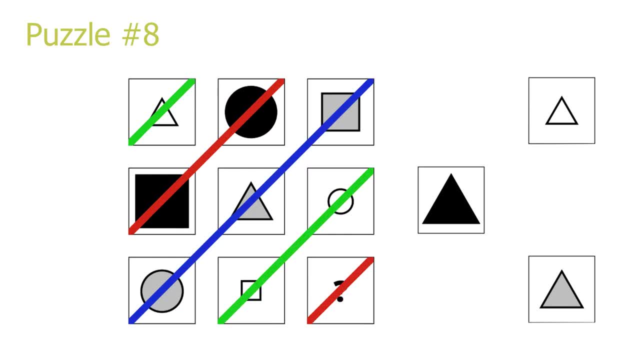 This leaves 2,, 3 or 6 as the correct answer. On the top right to bottom left diagonal, we have a repetition of color and size. On the red diagonals we have big shapes which also are black. This leaves our answer being a big black triangle. 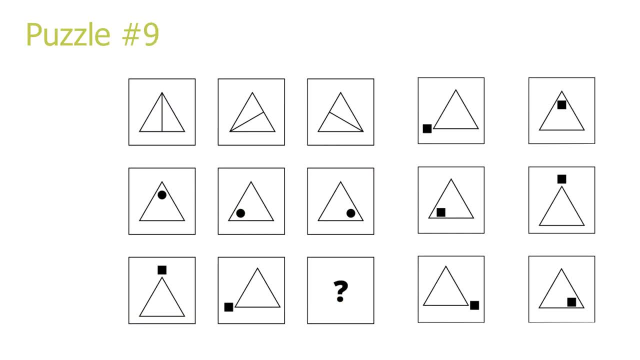 3 is the correct solution. Puzzle 9.. This is a row puzzle. If we look at one specific row- for example, let's start by looking at the first row- We see that the second picture is just the first picture, rotated 120 degrees counterclockwise. 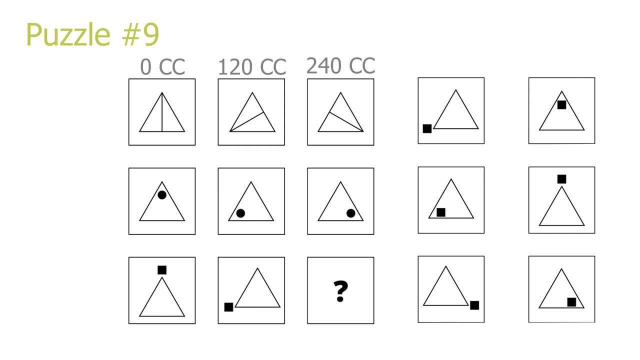 And then picture 3 is just picture 2, rotated 120 degrees counterclockwise. So, basing ourself on the third row, we can take picture 8 and rotate it 120 degrees counterclockwise to get our answer. 5 is the correct solution. 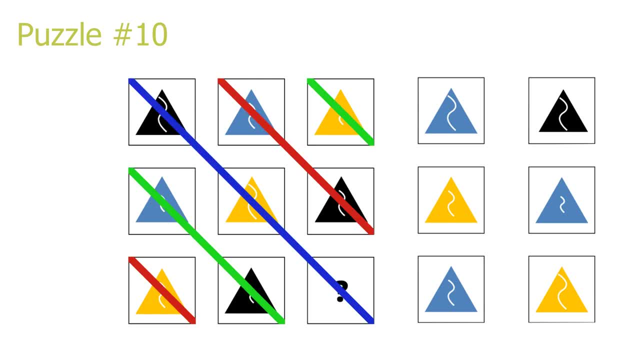 Puzzle 10.. This is a diagonal puzzle. On the top left to bottom right diagonal, we see that the shapes inside of the triangles repeat. On our main blue diagonal we have the biggest S shape leading to 1,, 2 or 6 as the correct. 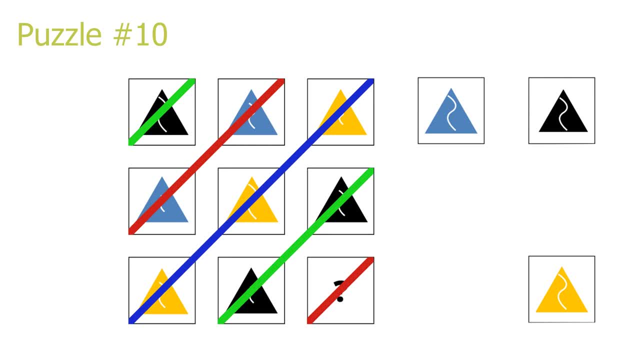 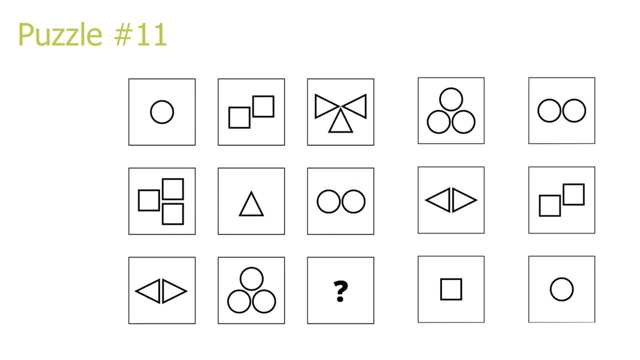 answer. On the top right to bottom left diagonal we see that the color inside of the triangles repeat. On our red diagonal we have blue repeating leading to 1 as the correct solution. Puzzle 11. This is another diagonal puzzle. On the top left to bottom right diagonal we have a repeating number of shapes. 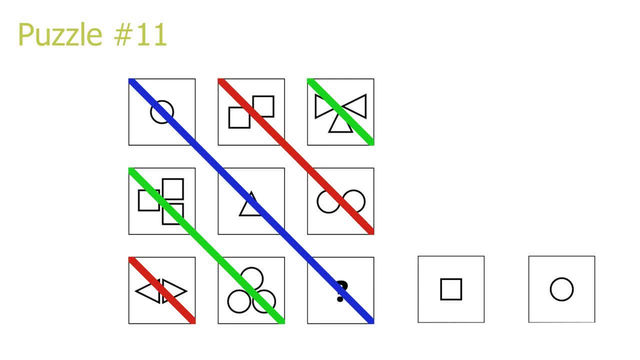 On the main blue diagonal, we have one shape repeating leading to 5 or 6 as the correct solution. On the top right to bottom left diagonal, we have repeating shapes. For the red diagonal, we have squares leading to our answer being a single square. 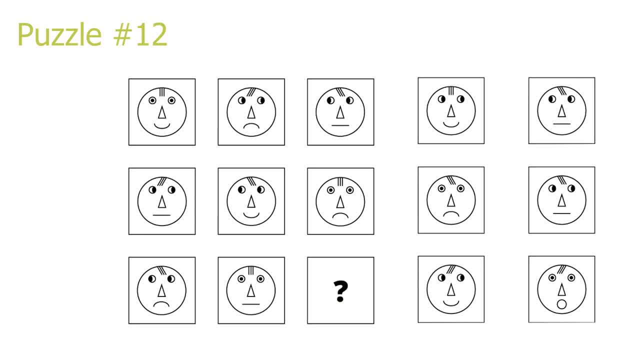 5 is the correct solution. Puzzle 12. This is another diagonal puzzle. On the top left to bottom right we have a repetition of the mouths. On the main blue diagonal we have the smiling mouth leading to 1 or 5 as the correct answer. 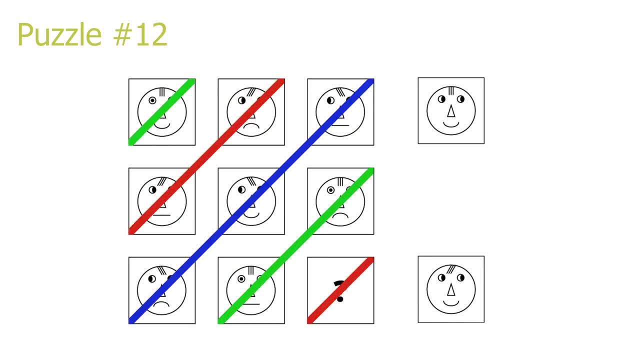 Puzzle 12.. This is another diagonal puzzle. On the top right to bottom left diagonal we have a repetition of the hair and eyes. Our answer is in the red diagonal leading to 5 as the correct solution. Puzzle 13.. This is a row puzzle. 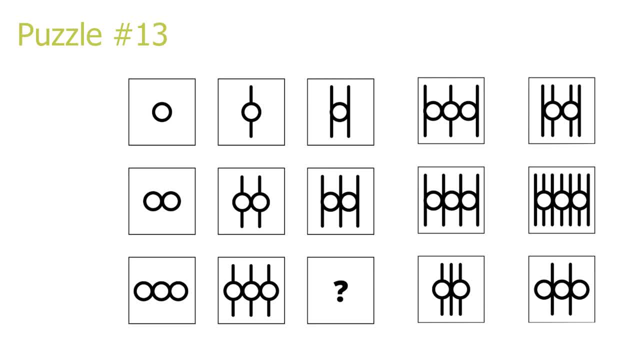 If we look at a specific row, for example row 1,, then we see that the second picture is just the first picture, with a vertical line added which go through the center of the circle, And the third picture is just the first picture with vertical lines added on the side of the. 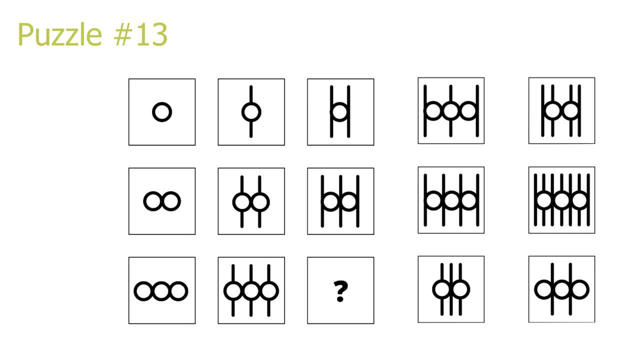 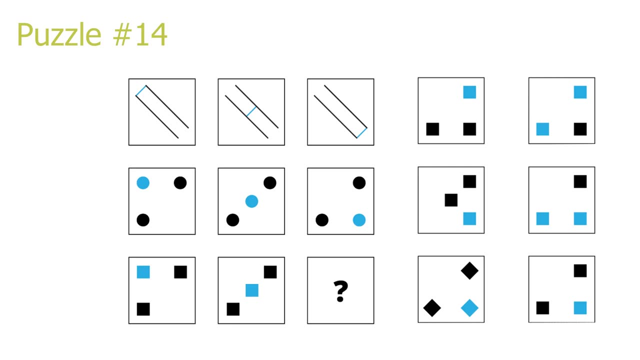 circles. So we have 3 circles and if we add one line on each side of these circles, we get our answer. This leads to 3 as the correct solution. Puzzle 14. This is a row and column puzzle. The easiest way to solve this one is just to base ourselves on the pictures in row 2. 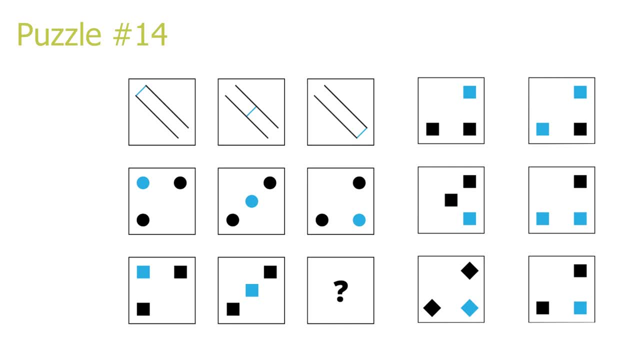 and change the circles into squares, which creates row 3.. So, basing ourselves on picture 6, we can convert the circles into squares in order to get our answer. Answer 6 is the correct solution. Puzzle 15.. This is a row and column puzzle. 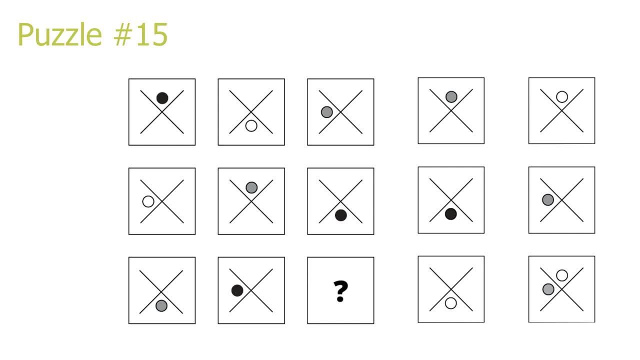 This is a diagonal puzzle. First, if we look at the top left to bottom right diagonals, we have a repetition of the circles placement. On the main blue diagonal we have the circle on top repeating leading to 1 or 2 as the. 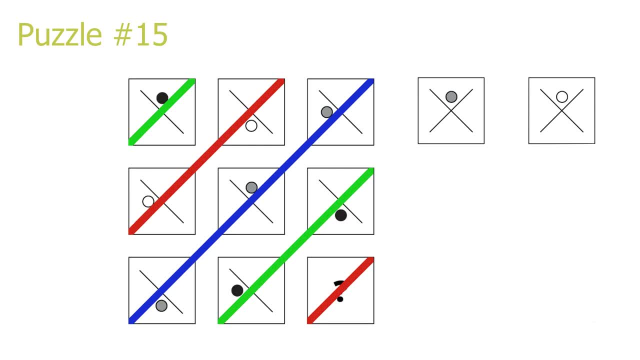 correct answer. On the top right to bottom left diagonal we have a repetition of the color inside of the circle. On the red diagonals we have a repetition of white inside of the circles. This leads to our answer having a white circle on top. 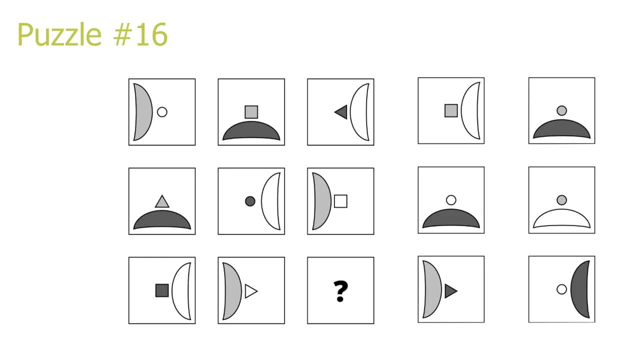 2 is the correct solution. Puzzle 16.. This is another diagonal puzzle. On the top left to bottom right diagonals there is a repetition of the shape in the middle of the pictures. In the main blue diagonal there is a repetition of the circle in the center. 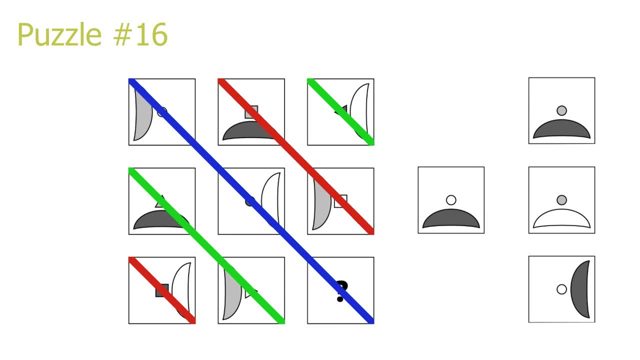 This leads to 2,, 3,, 4 or 6 as being the correct solution. On the top right to bottom left diagonals, there is a repetition of color and orientation of the half circle. On the red diagonals, the half circle is on the bottom. 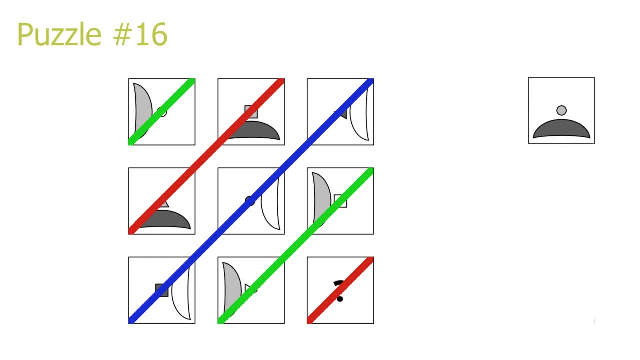 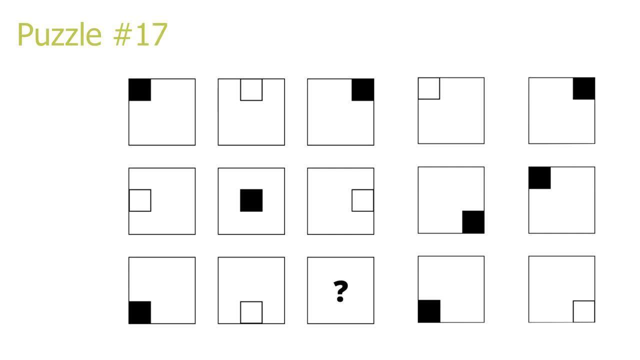 The half circle is dark grey and the circle in the middle is light grey- Puzzle 17.. This is the correct solution. Puzzle 17.. This is a kind of symmetry puzzle. First, let's look at the repetitions in the columns. We see that there are only squares in the columns where the lines I've drawn in are. 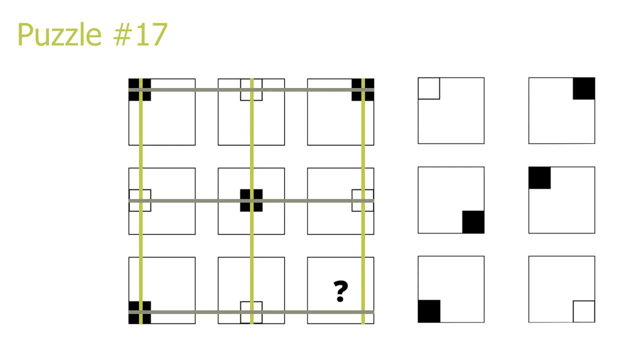 On the rows. we have the same thing and we can see how there are only squares in the intersection between these two lines I've drawn in. We also have this X shape in the middle where all the squares are black. Therefore, we know that our answer is a black square in the bottom right corner. 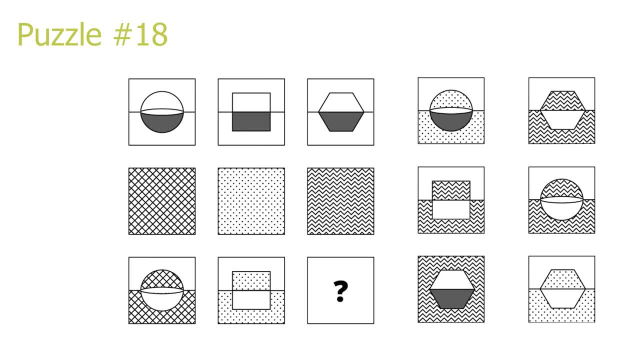 4 is the correct solution. Puzzle 18.. This is a column puzzle, So in order to figure out how to get the third picture in a column, let's look at the first column as an example. We see that the third picture and the first picture in column 1 is very similar. besides, 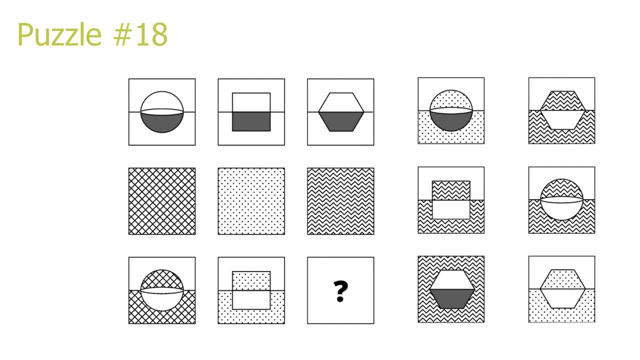 three things. In the third picture the bottom half of the circle shape has been turned from dark grey to white. The top half of the circle shape has been turned from white to the pattern in picture 2 in the column And the bottom half of the main square shape has been turned from white to the pattern. 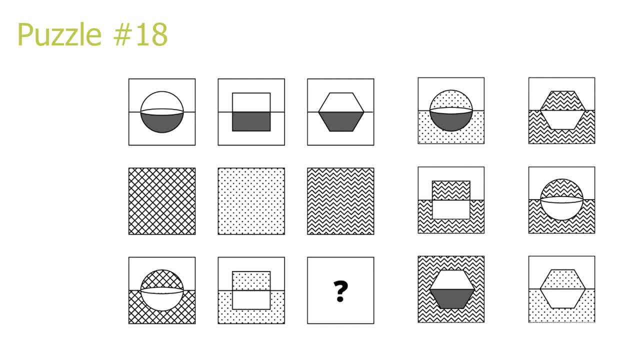 in the second picture in the column. The same pattern repeats for the second column. So we just have to do the same for the third column. We take the first picture in the column and remove the dark grey area and then add the pattern of the second picture in the column on the top half of the hexagon and on the 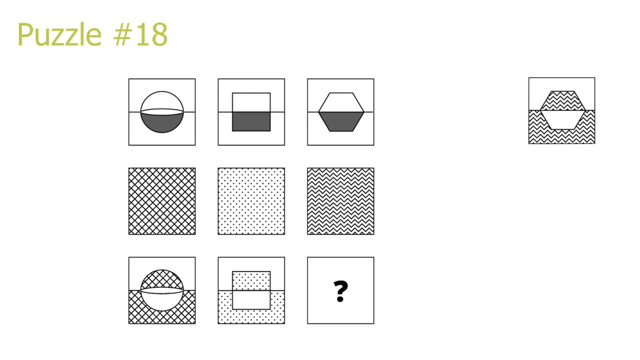 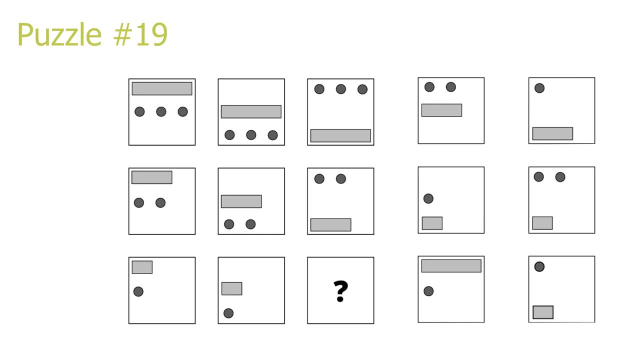 bottom half of the main square shape. This leads to 2 as the correct solution. Puzzle 19.. This is our one column puzzle. If we look at column 1, we see that if we take picture 1 and remove the right, most column 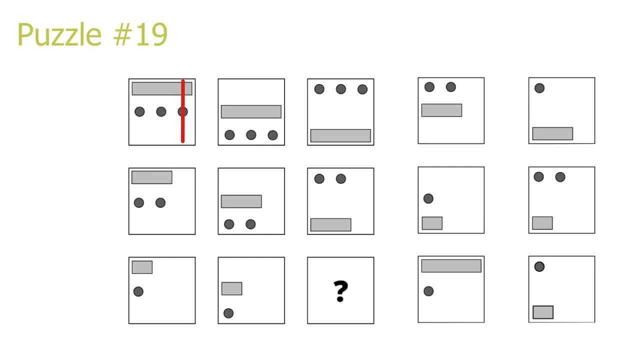 then we get picture 2.. And if we take picture 2, we get picture 1.. 2 and remove the rightmost column, we get picture 3.. The same holds up for column 2, so we can use this to solve the puzzle. 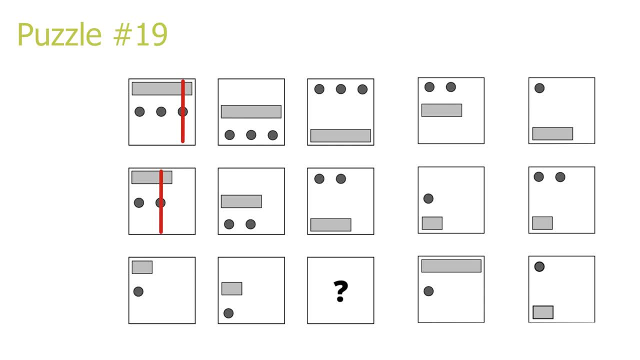 So if we look at the third column, then we get the second picture from removing the rightmost column in the first picture and we will get our answer if we take the second picture and remove the rightmost column, leading to 6 as the correct solution. 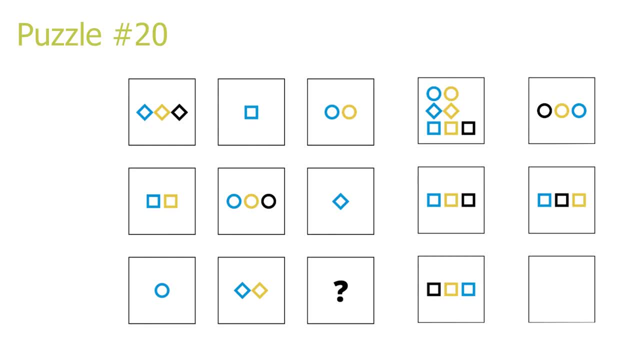 Puzzle number 20.. This is a diagonal puzzle on both diagonals. First, if we look at the top left or bottom right diagonal, we see that the number of shapes repeat. On our main blue diagonal we have 3 shapes. This leads to 2,, 3,, 4 or 5 as the correct solution. 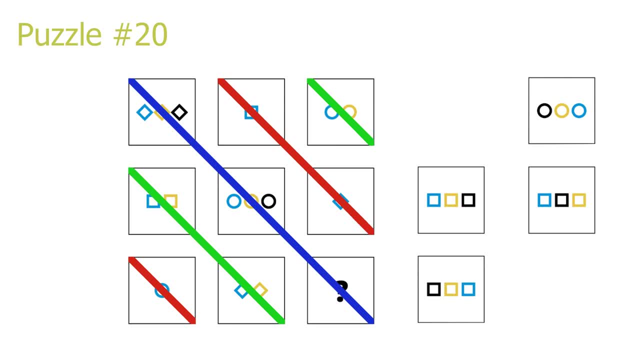 We can also see that the color pattern among these diagonals repeat. So on our main blue diagonal we have blue, yellow, black in that order from left to right. This leads to 3 as the correct solution. Puzzle 21.. This is another diagonal puzzle. 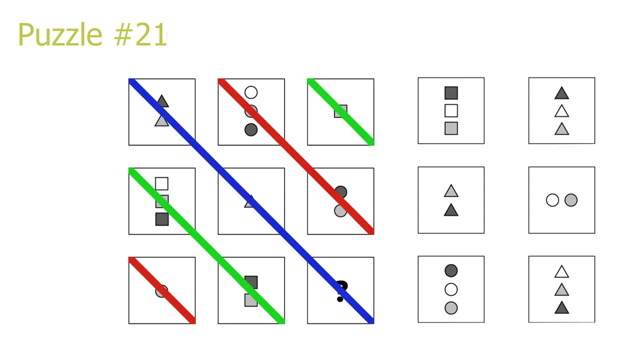 If we look at the top, left or bottom right diagonal, we see what kind of shape repeats. For the main blue diagonal, the triangle shapes repeat. This leaves 2,, 3 or 6 as the correct answer. On the top right to bottom left diagonal, we see that the amount of shapes and the order 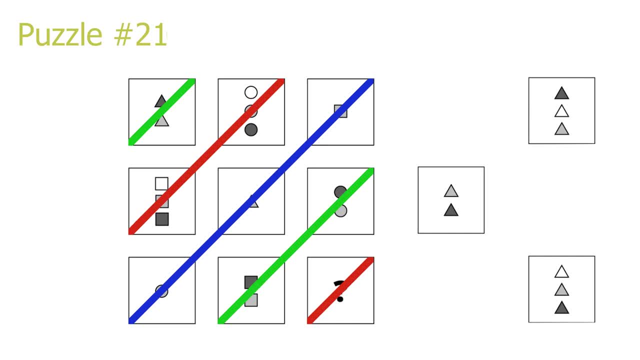 of the color repeats. On the red diagonals we have 3 shapes with the color of white, grey and black from top to bottom. This leaves 6 as the correct solution, Puzzle 22.. So the first thing to notice about this puzzle is that on the columns, the small shapes inside. 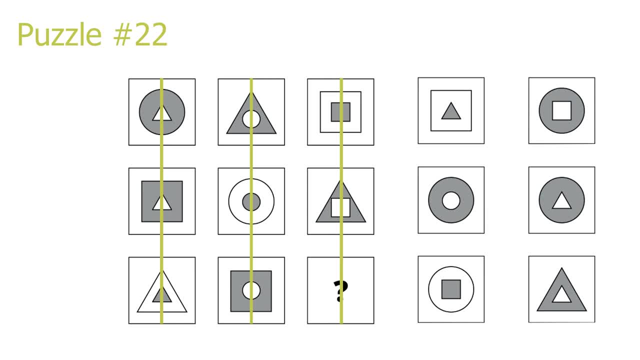 repeat On the last column we have squares inside leading to 2 or 5 as the correct answer. This leaves 6 as the correct solution. Puzzle 22.. On the top right to bottom left diagonals, we see how the blue diagonals have a white. 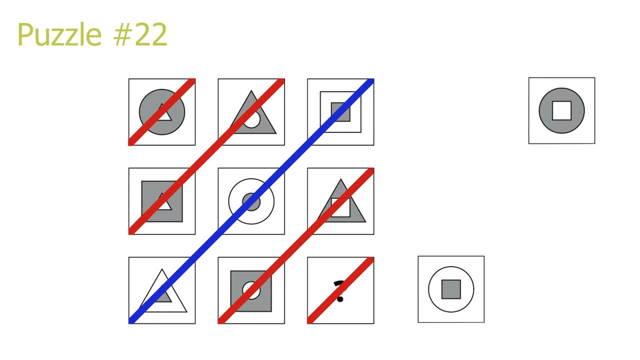 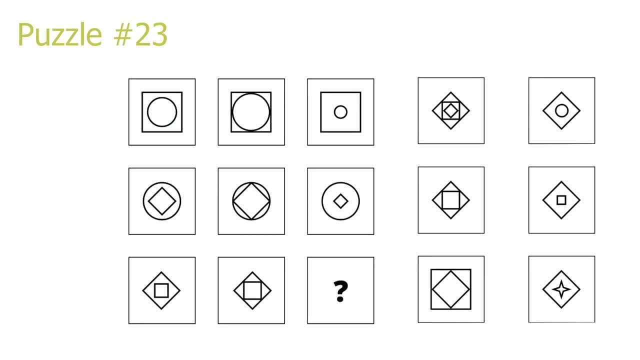 main shape and a grey smaller shape, while the red diagonals, which our answer is in, has a grey main shape and a white smaller shape. This leads to 2 as the correct solution. Puzzle 23.. This is our one column puzzle. I solved it by looking at the rows. 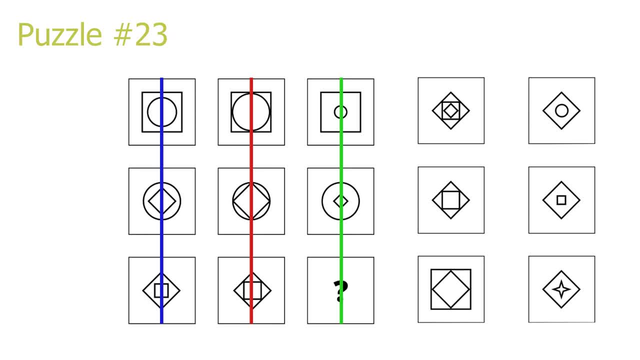 We can see how the inside shape changes in size when moving from column to column. In the first blue column the inside shape is second smallest, In the second red column it's biggest and in the third green column it's smallest. Since the third column has the smallest inner shapes, we know that the square inside of our 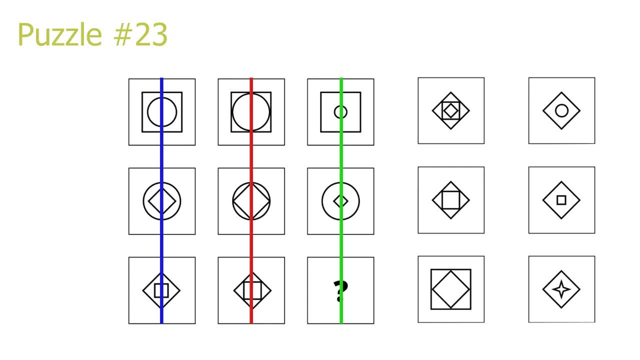 answer has to be smaller than the square inside of the first picture in the third row. Only one answer has such a small square and it's answer 4.. Puzzle 24.. This is the final puzzle of the test. First, if we look at the rows, we have a 45 degrees clockwise rotation when moving from. 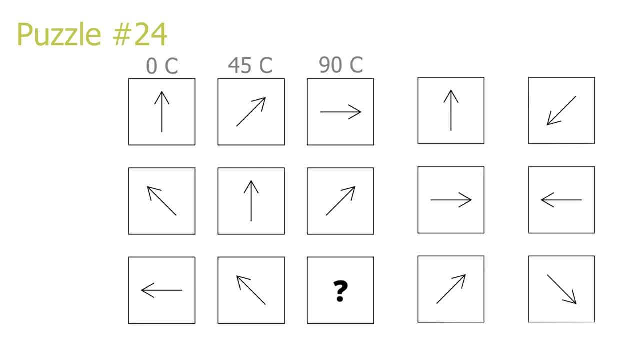 one picture to the next picture, So we can base ourselves on the last row, and taking picture 8 and rotating it 45 degrees clockwise leads to an arrow pointing upwards. One is the correct solution. We could also have solved this easily by the columns where we have a 45 degrees counter. 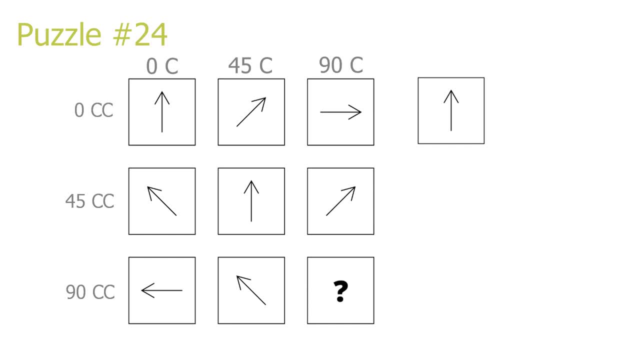 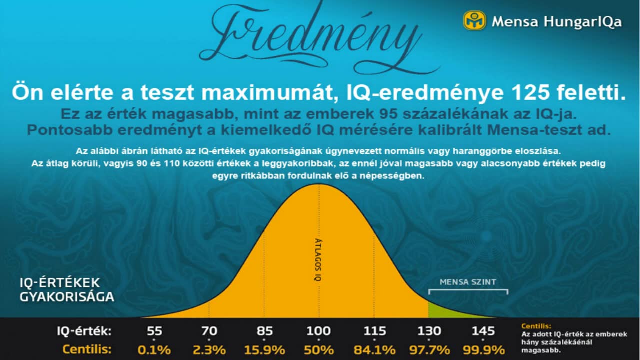 clockwise rotation. This also leads to an arrow pointing upwards. So here is the final result when I took the test. I'm assuming that most people watching this will have no clue what it says, including myself, so I translated the text: Yes, you have reached the maximum score of the test. 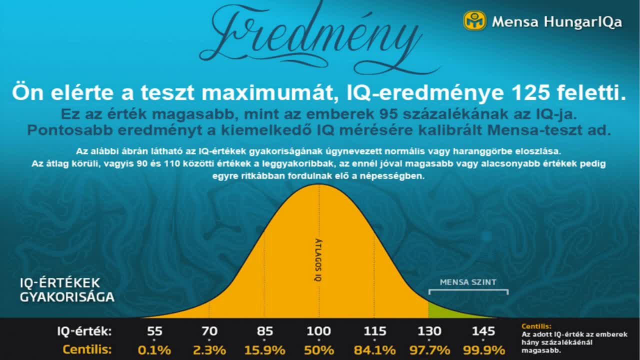 Your IQ score is above 125.. And then the rest of the text just says how a real Mensa IQ test is more accurate. As always, I hope you enjoyed the video and I'll see you again in the next puzzle. 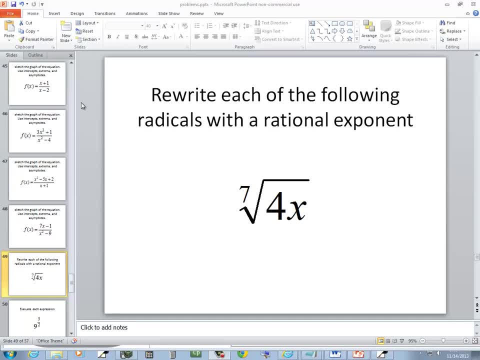 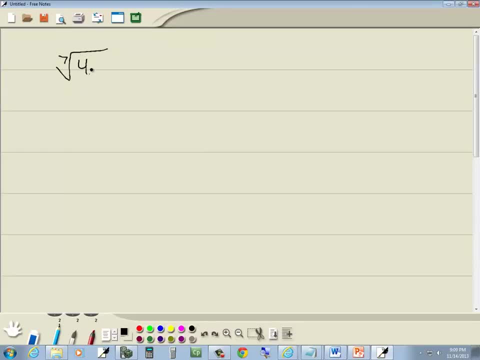 In this problem. we want to rewrite each of the following radicals with the rational exponent fractional power. So we've got 7th root of 4x. Well, I can rewrite this as the 7th root of 4x to the 1st power. 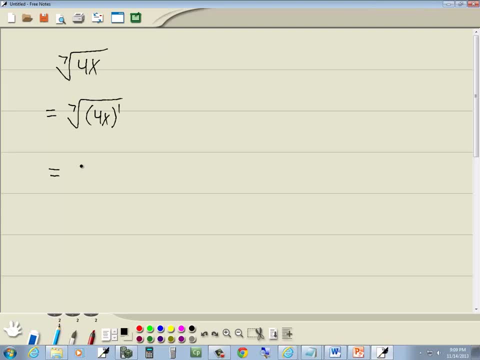 Now to rewrite this in rational exponent form or fractional power. this is going to be 4x to the 1- 7th power, Whatever power is inside here, and there's always an implied 1 if you don't have any power. 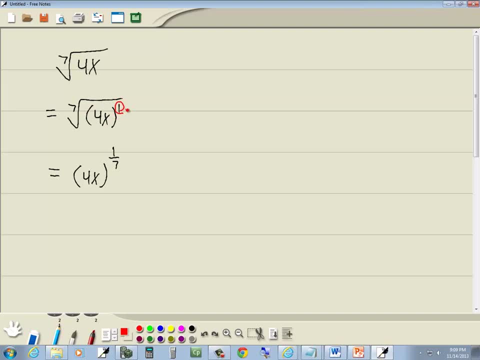 but the entire inside of the radical has to be to that power. That's what goes up on top. Now, whatever number is in our slot right here, that's called our index. That's what goes down in our denominator. So that's how we get 4x, all of it to the 1, 7th power.